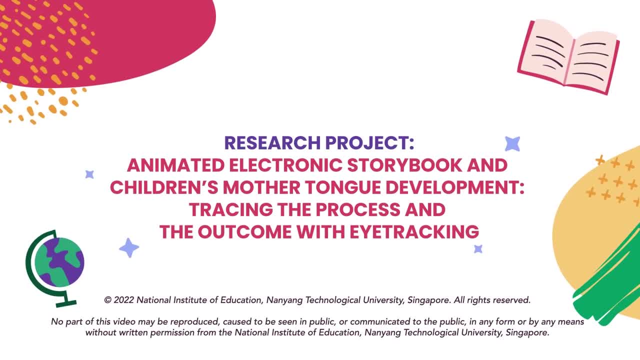 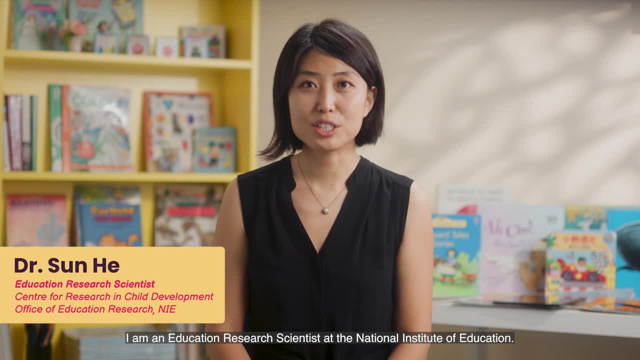 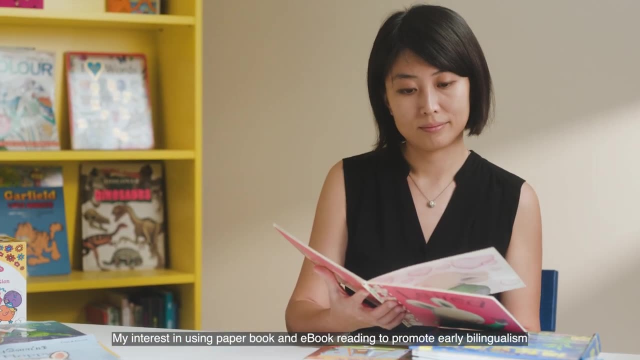 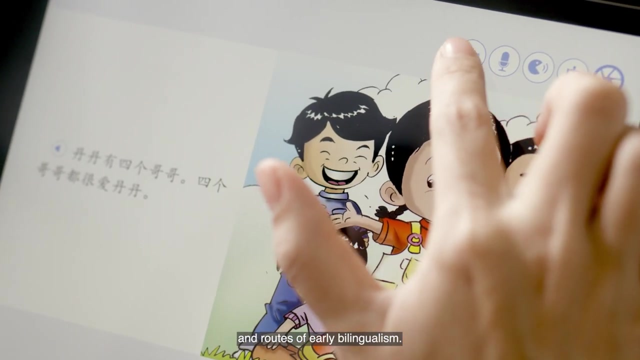 Hello everyone, my name is Sun He. I'm an education research scientist at the National Institute of Education. My interest in using paper book and e-book reading to promote early bilingualism started from how cognition and environments co-shape the developmental rates and roots of early bilingualism. Bilingualism is the cornerstone of Singapore's education. 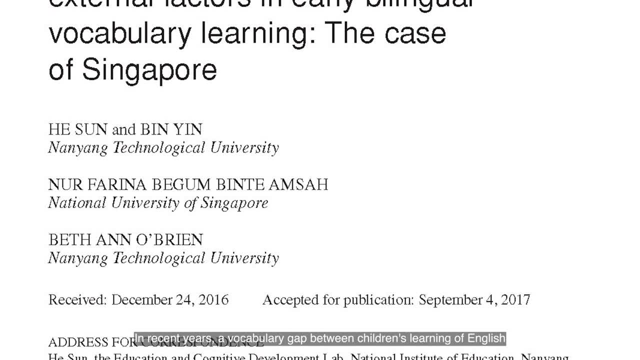 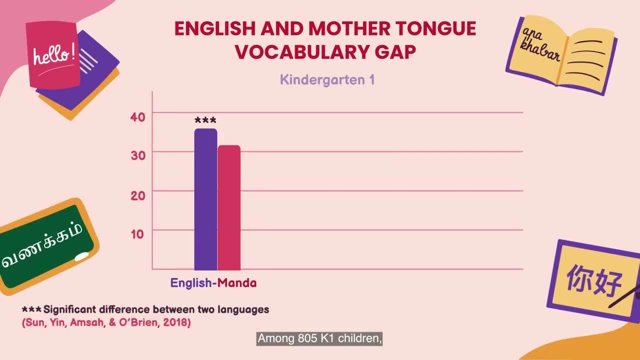 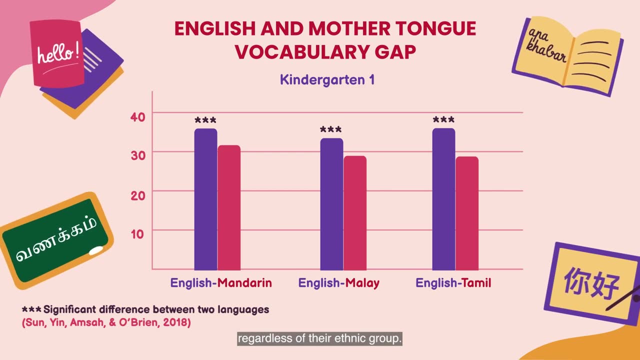 In recent years, a vocabulary gap between children's learning of English and mother tongue language is observed. Among 805K1 children, they were found to have larger English vocabulary size than their mother tongue vocabulary, regardless of their ethnic group, And we know that. reading. 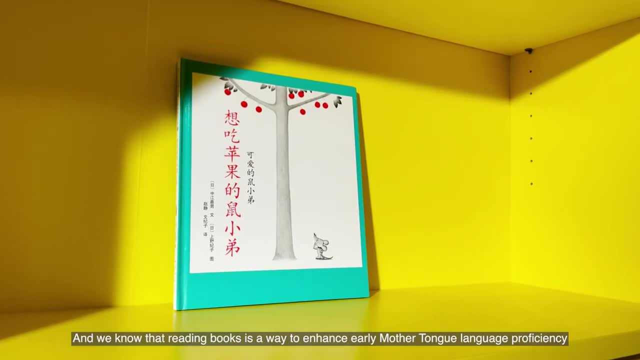 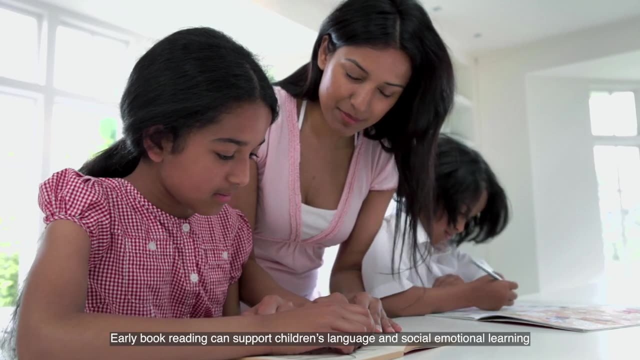 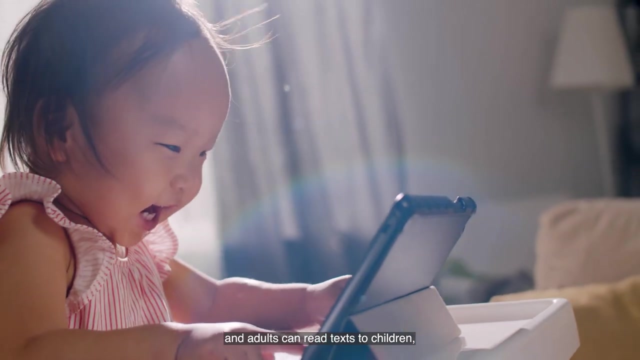 books is a way to enhance early mother tongue language proficiency and it has lasting effects on children's development. Early book reading can support children's language and social-emotional learning and other domain development, And adults can read texts to children, ask them questions and 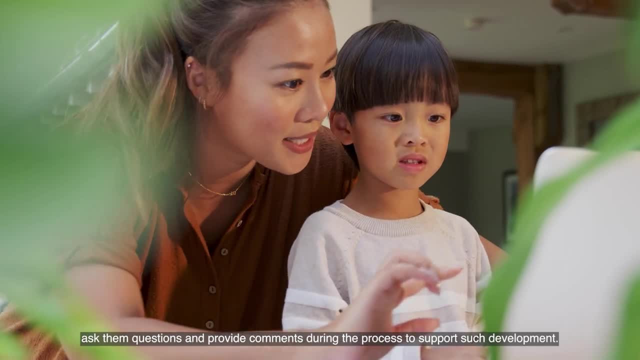 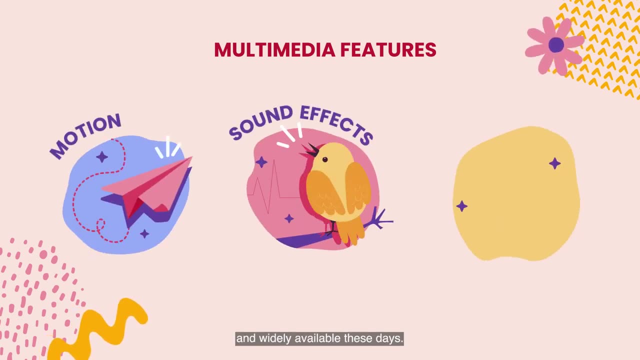 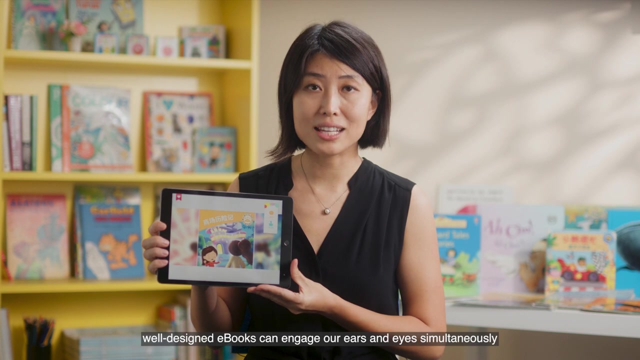 provide comments during the process to support such development. E-books or books that have multimedia features are very popular and widely available these days. According to the multimedia theory, well-designed e-books can engage our ears and eyes in a new world. We use e-books simultaneously to process the reading materials by reducing our cognitive. 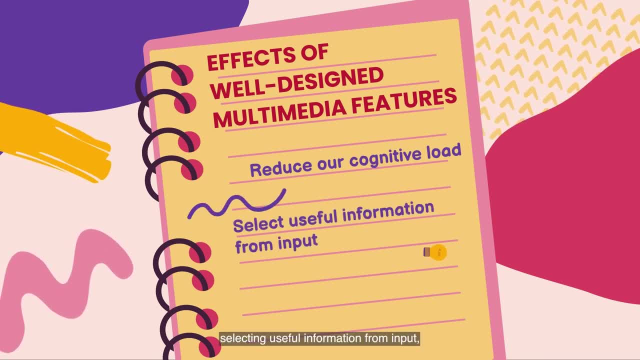 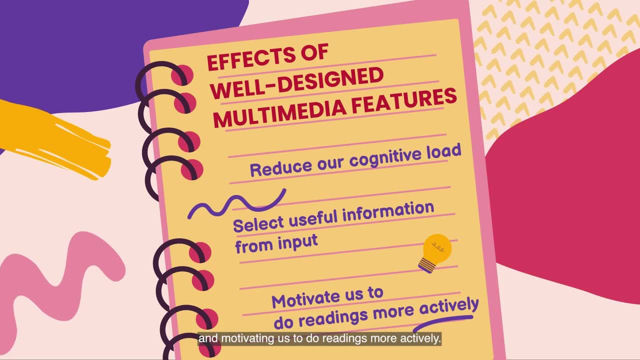 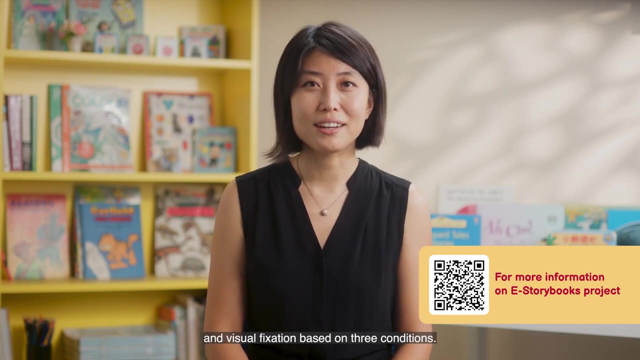 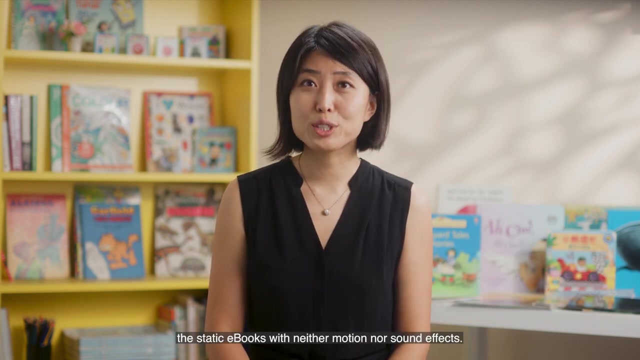 load, selecting useful information from input and motivating us to do readings more actively. We explore the effectiveness of animated e-books on children's Mandarin learning outcomes and visual fixation based on three conditions. Number one: the static e-books with neither motion or sound effects. 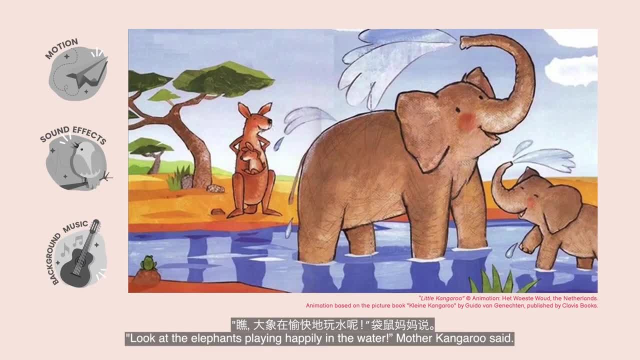 Number two: the static e-books with neither motion or sound effects nor sound effects. 瞧大象在愉快地玩水呢袋鼠妈妈说。. Two, the static e-books with no motion but with sound effects. 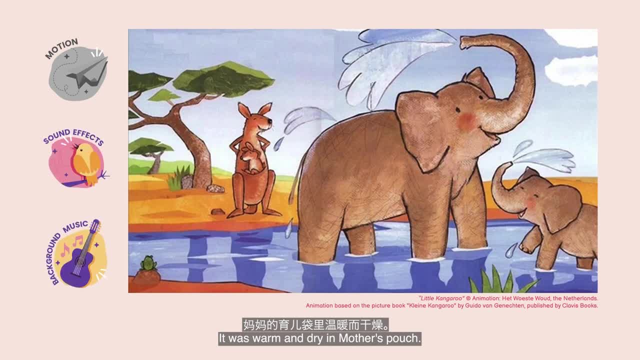 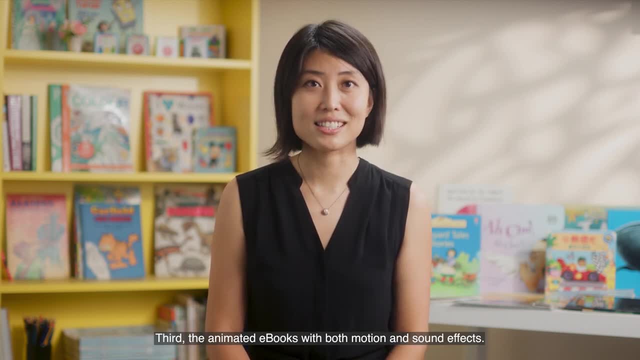 妈妈的育儿袋里温暖而干燥。. Third, the animated e-books with both motion and sound effects. 听到鸟叫我都想跳舞了。. 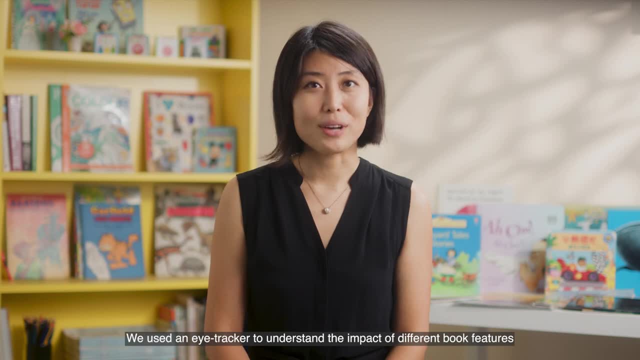 你想跳舞吗宝贝? We use an eye tracker to understand the impact of different e-book features on children's eye fixation during reading, For example, what features they fix their eyes on and how long they do so. 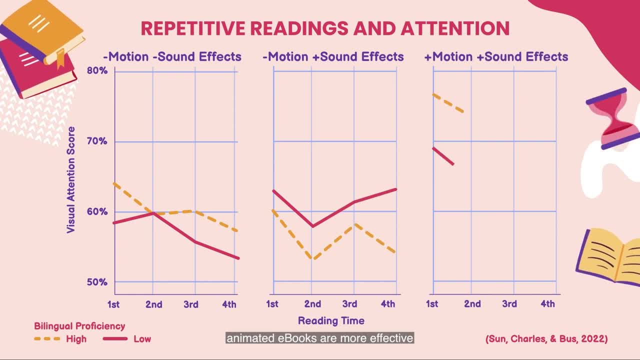 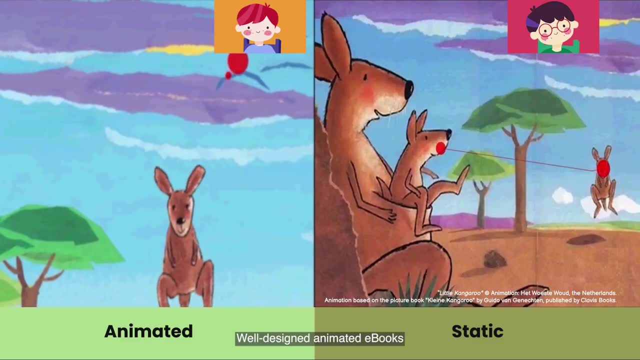 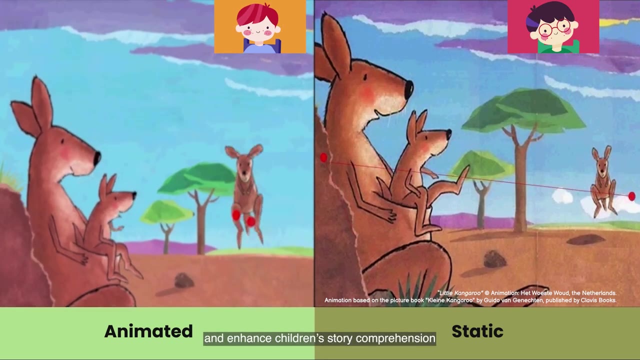 Overall, the current study shows that animated e-books are more effective in holding children's attention than static e-books. Well-designed animated e-books help to direct children's attention to the rich details of the story and enhance children's story comprehension and word learning. 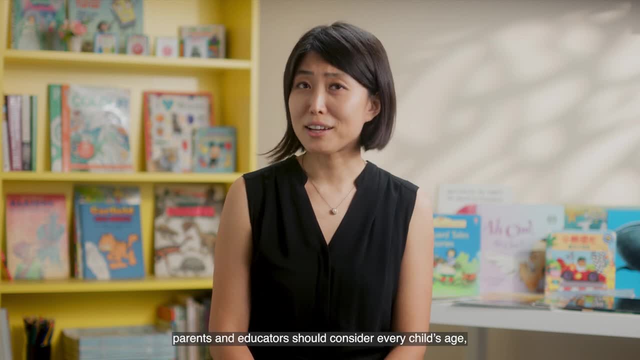 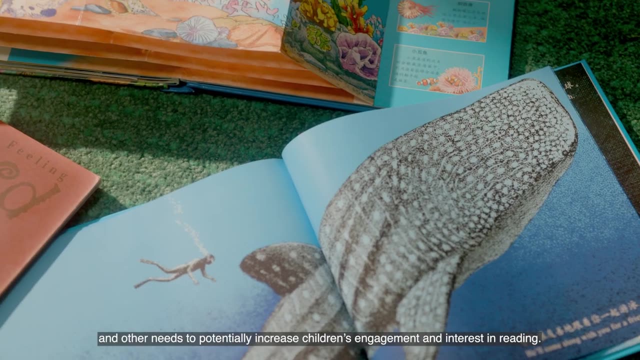 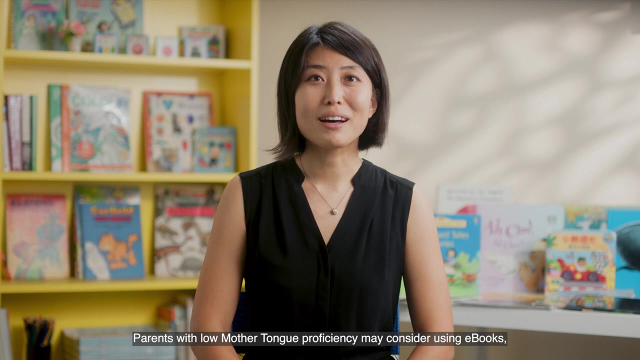 Just like a printed book. parents and educators should consider every child's age, developmental stage, interest and other needs to potentially increase children's engagement and interest in reading. Parents with low mother tongue proficiency may consider using e-books, especially the reading aloud function. 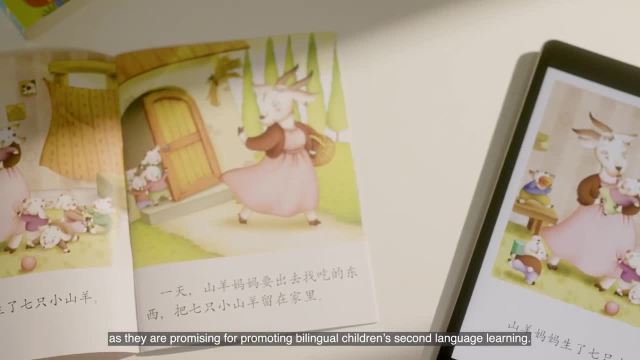 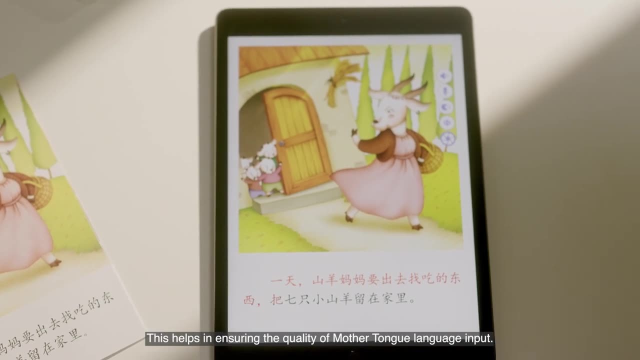 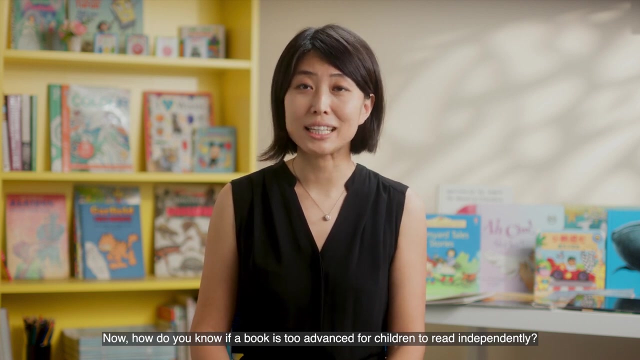 as they are promising for promoting bilingual children's second language learning. This helps in ensuring the quality of mother tongue language input. Now, how do you know if a book is too advanced for children to read independently? A good way to remember is the five-finger rule. 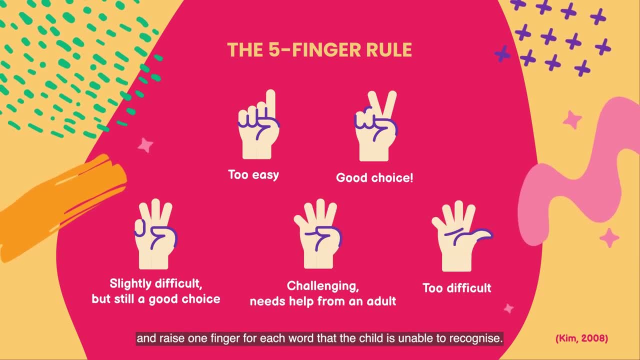 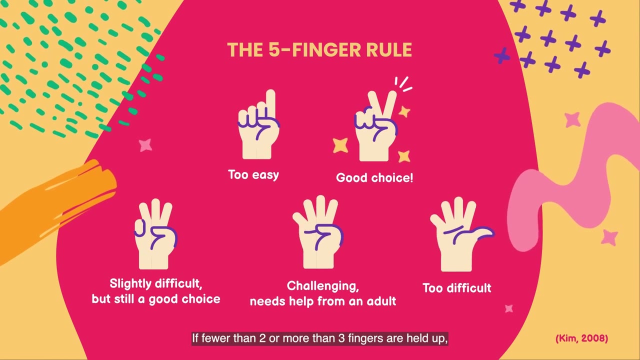 Open the book to any page and raise one finger for each word that the child is unable to recognize. An ideal book will be one with a single finger, One where only two to three fingers are held up. If fewer than two or more than three fingers are held up, 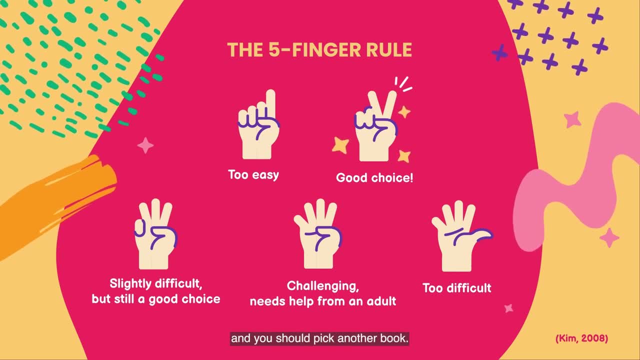 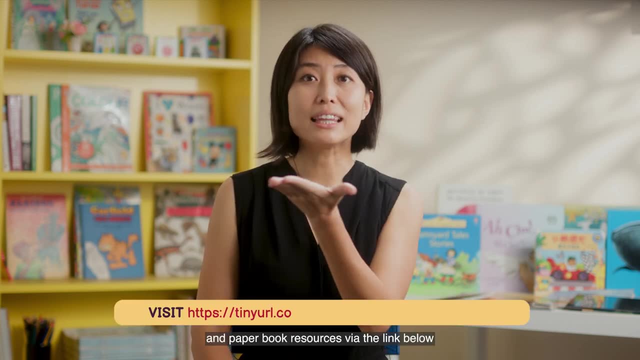 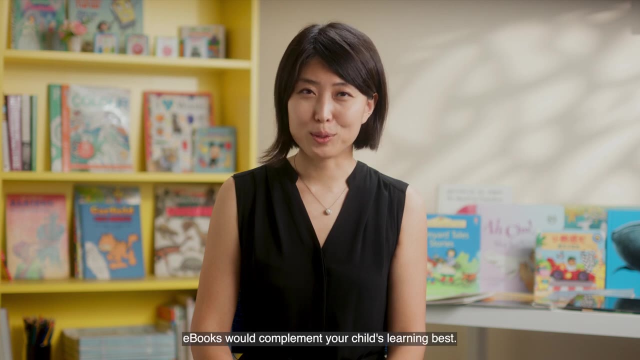 the book is either too easy or difficult and you should pick another book. You can access good e-books and paper book resources via the link below. Make use of these website's features to decide which e-books would complement your child's learning best. 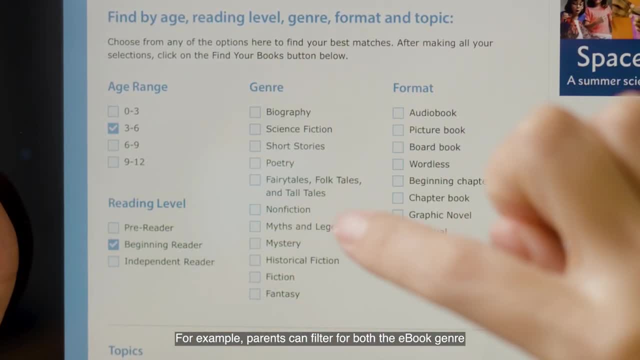 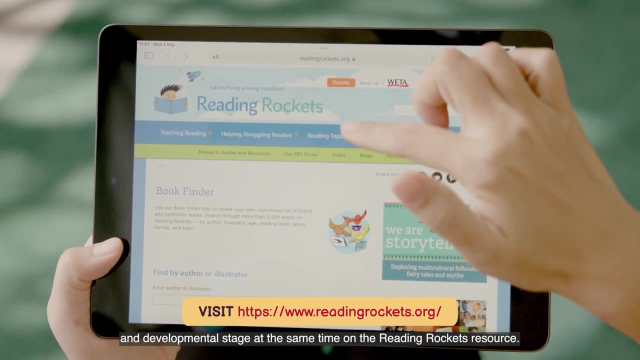 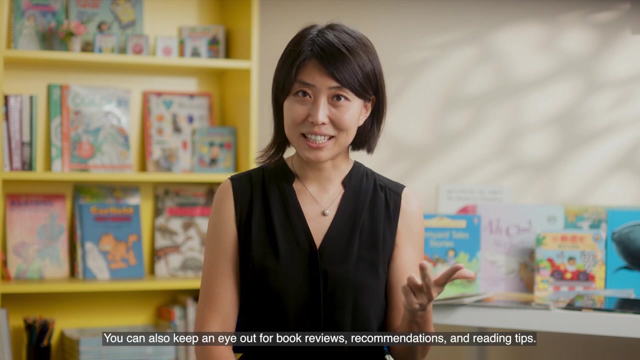 For example, parents can filter for both the e-book genre and developmental stage. at the same time, on the Reading Rocky resource, You can also keep an eye out for book reviews, recommendations and reading tips to gain more tips on bilingualism beyond reading e-books.